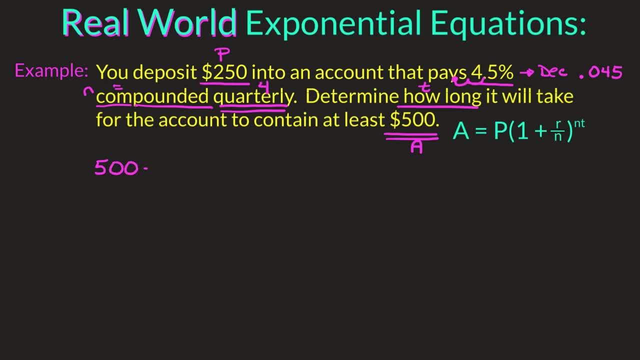 have. A was 500. So 500 equals our P was 250.. So 250 open parentheses, one plus our rate is 0.045 divided by our N Value, which we decided was four. Close parentheses to the four for N times our T, which we do not. 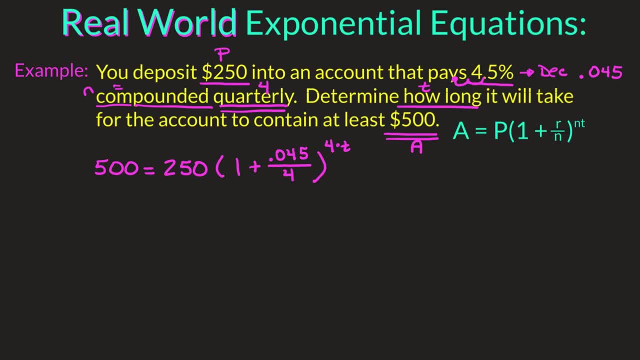 know That's what we're trying to solve for. Okay, So to get the T by itself, we need to divide both sides by 250. And when we do that, the 250s cancel. 500 over 250 gives us two, So we have two. 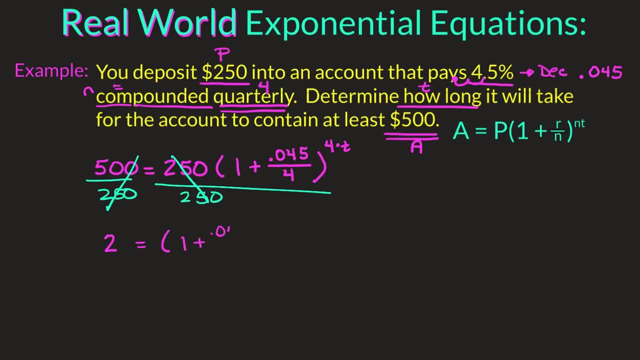 equals parentheses, one plus 0.045.. Over four Close parentheses to the four T power. Now, when we do this, I want to- I do a couple of different ways sometimes, But if you can plug in what's in the parentheses into your calculator and it will give you not too long of a decimal, then I say, go ahead and simplify it further And in this case it does give us some decent decimal. So we have two equals parentheses, one point zero, one, one, two, five. 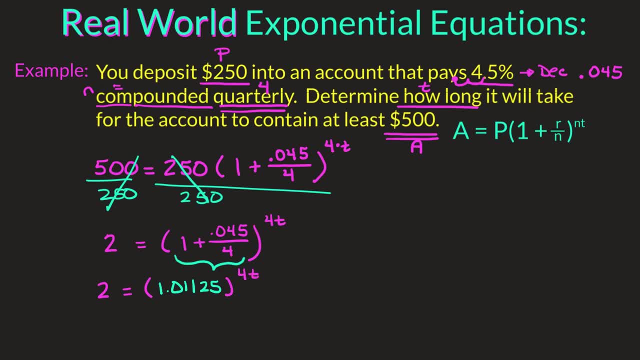 Close parentheses to the four T power. Now that parentheses is now your base And so now we're going to have to log base both sides. So we're going to log base one point zero, one, one, two, five on both sides, because we want those to cancel. 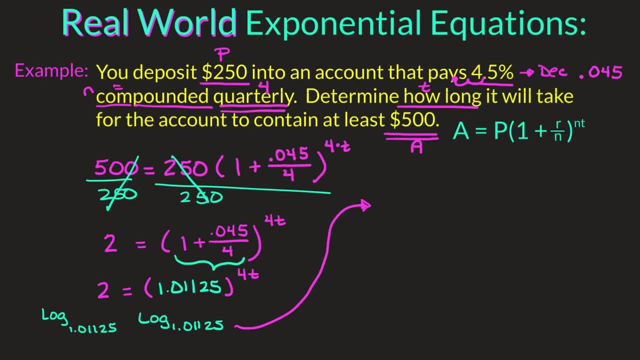 So I'm going to continue writing over to the side a little bit so I have more room. So the first, the left side. we're going to have log base one point Zero, one, one, two, five of two equals the log base and the base will cancel and that's going to leave us with four t from here. You still need to get to you by itself. So you're going to divide both sides by four and that's going to leave us with 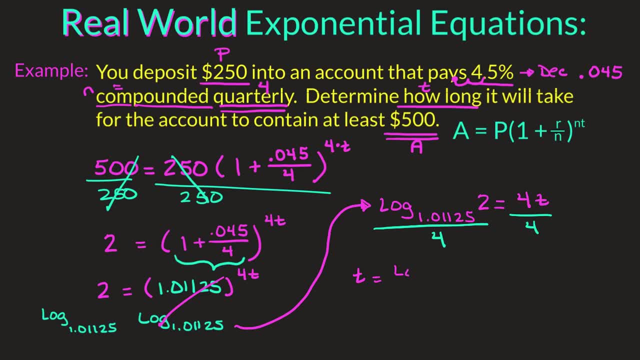 T Equals Log Base: one point zero, one, one, two, five of two all over four. Then plug that information into your calculator and get the value once you hit enter, And that will be our approximate amount of time. So T will be approximately 15.489.. 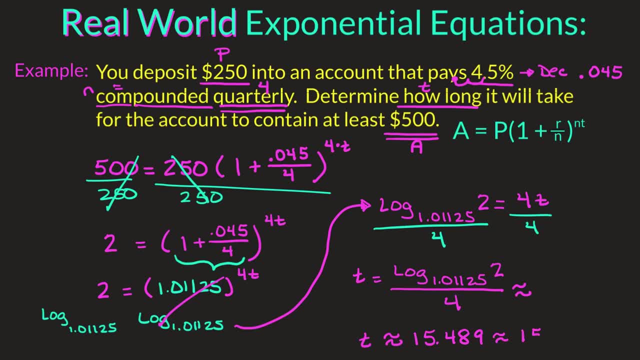 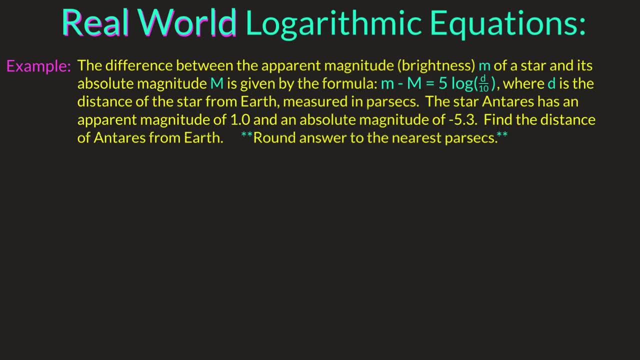 Let's simplify that to approximately 15.5 years for our money to double. Here we are with our last real world log problem. So it says the difference between the apparent magnitude or the brightness, is lowercase m of a star And its absolute magnitude, uppercase M or capital M, is given by the formula: lowercase m minus capital M equals 5 times the log of d divided by 10.. 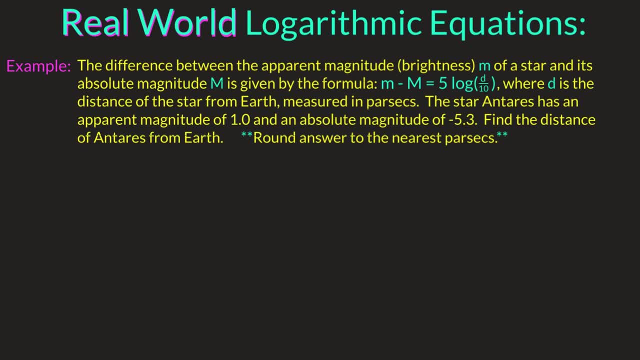 Where d is the distance of the star from the earth measured in parsecs. The star in Taurus has a. It has an apparent magnitude. So apparent magnitude, And up here it mentions that apparent magnitude is the lowercase m. So we know that this is M. 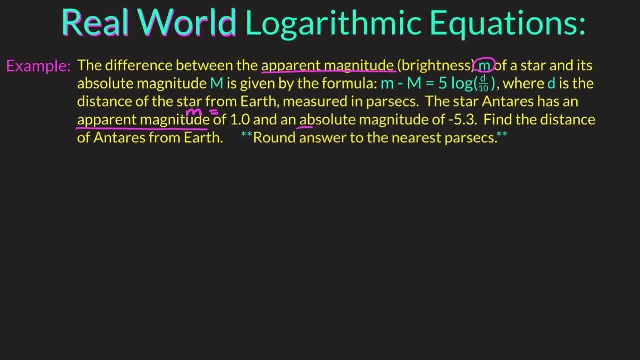 It's going to equal 1.0.. And it has an absolute magnitude. An absolute magnitude is mentioned up here. It says it's represented by the capital M. So that will be our uppercase. M is negative 5.3.. Find the distance of the star. 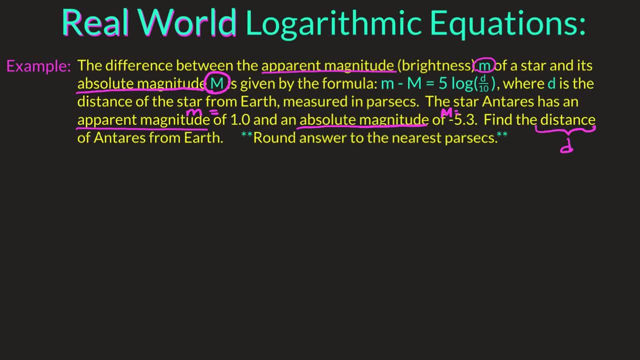 So this is what we're looking for. We're looking to find d of Antares from earth And it says round, our answer to the nearest parsecs. So let's plug in our information that we're given and solve for the unknown. So our lowercase m, we said, was 1.0, minus our uppercase M, or our capital M. 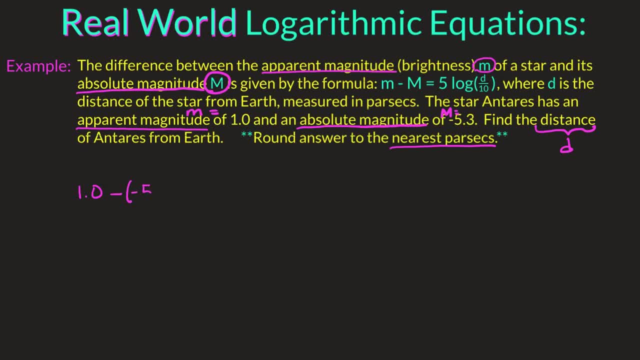 which is negative. 5.3, equals 5 times the log of d, which is distance. We don't know what that is Divided by 10, close parenthesis. So if we take a look at this, we're going to simplify where we can. 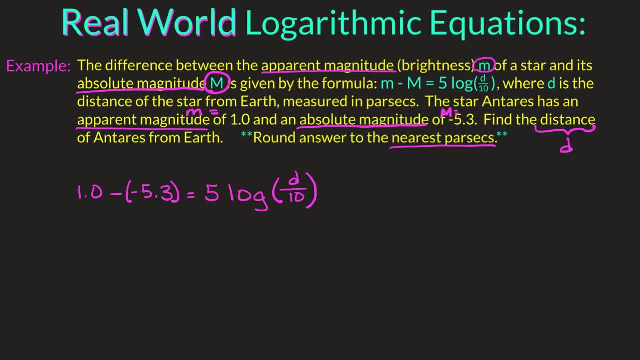 It looks like on the left side we can do a little bit of simplifying, So we have 1 minus a negative 5.3, which is actually 1 plus 5.3,, which gives us 6.3. Because a minus a negative is a plus. 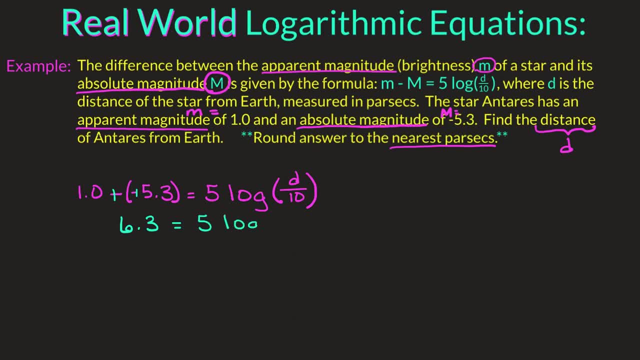 Equals 5 times the log of d divided by 10.. Now again, we're trying to isolate the log. So that means now we're going to divide both sides by 5.. The 5's will cancel And that gives us 6.3 divided by 5.. 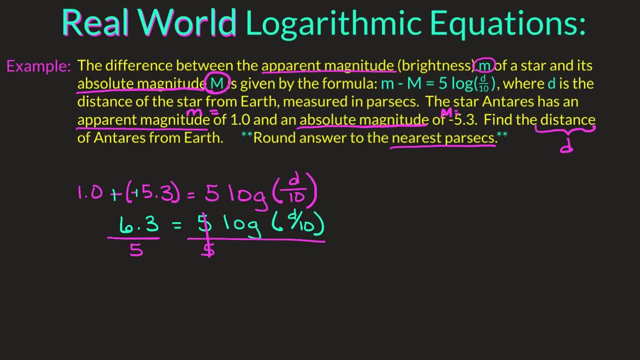 And that's going to give us 1.26.. So 1.26.. 1.26 equals the log of d over 10.. Now we need to get rid of this log. The only way to get rid of the log is to exponentiate both sides by the base of the log. 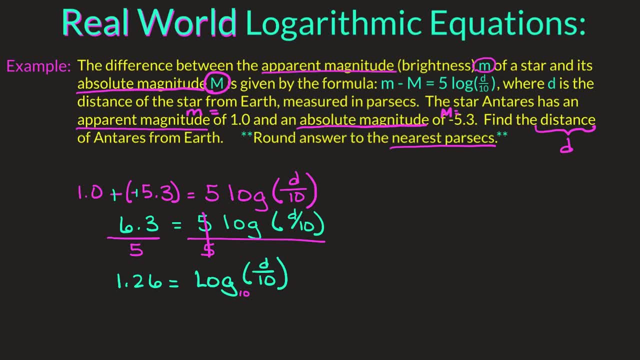 Our base of the log is not written but it's understood to be a 10.. So we're going to exponentiate using 10 on both sides. So now we have the 10 and log base 10 cancel. giving us 10 to the 1.26 power equals d divided by 10.. 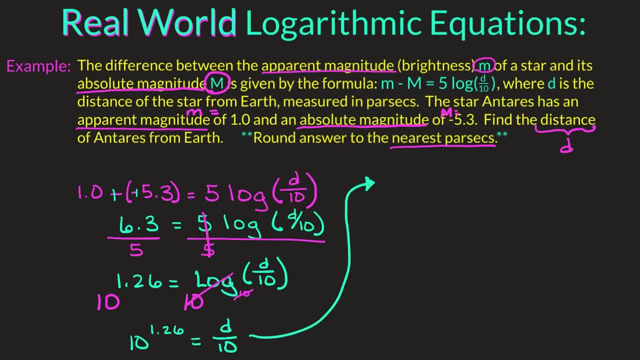 I'm going to go over to the side so we have a little bit more room to work And rewrite our problem. So we now have 10 to the 1.26 equals d over 10.. I'm going to go ahead and simplify the left side. 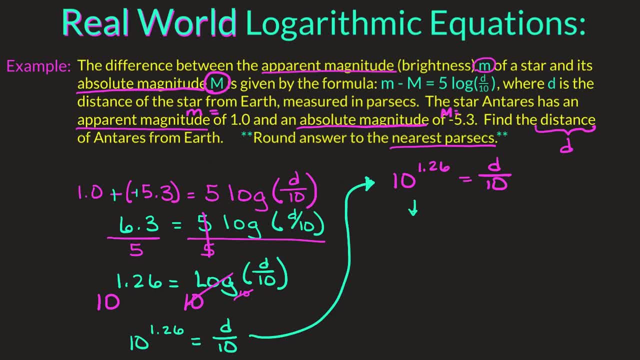 So we have 10 to the 1.26.. I'm plugging that in the calculator. It's going to be approximately. I'm going to go ahead and round to the nearest thousandth. So we have 18.197 equals d divided by 10.. 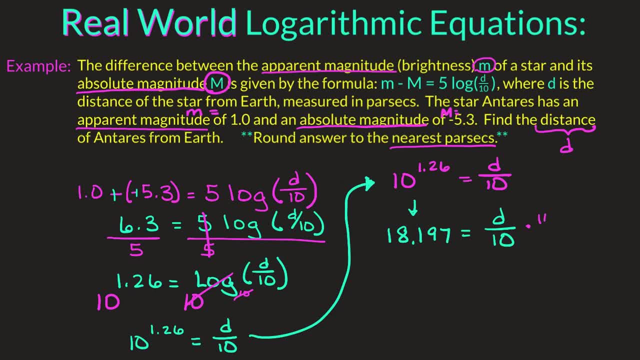 Here we can multiply both sides by the denominator And that will give us d by itself. So d equals 10 times our 18.26. Times our 18.197. Which would give us 181.97.. Our directions say to round to the nearest par 6..